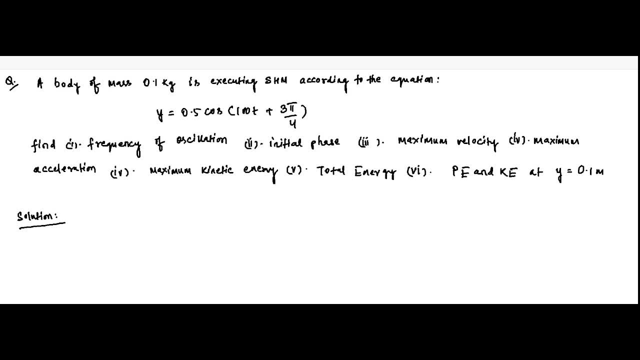 So here is another question on energy of an object or a body undergoing simple harmonic motion. So here it is given that a body of mass 0.1 kg is executing simple harmonic motion. according to the equation, y is equal to 0.5 cos 100 t plus 3 pi by 4.. But y is the 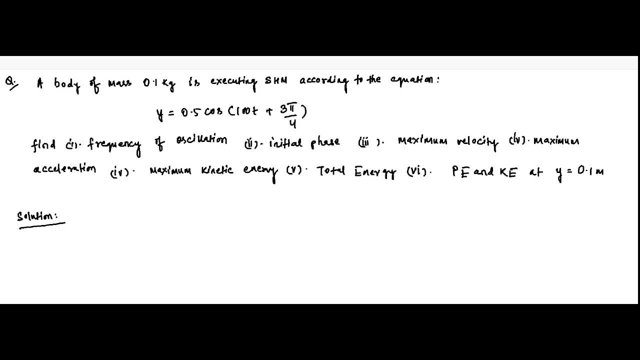 position of the object, the instantaneous position. We have to find the frequency of oscillation, the initial phase, maximum velocity, maximum acceleration, maximum kinetic energy, total energy and potential energy and kinetic energy at y is equal to 0.1 meter At this. 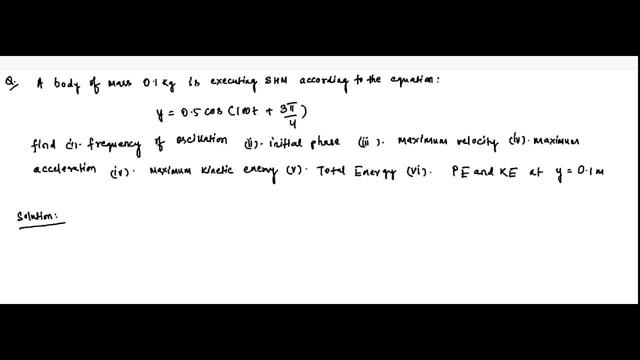 particular position, 0.1 meter, we have to find both potential and kinetic energy. Okay, So first, as usual as we do, first write this standard SHM equation format. It can be in sine or cos. Basically it is sinusoidal. So here we write it in cos, because the given 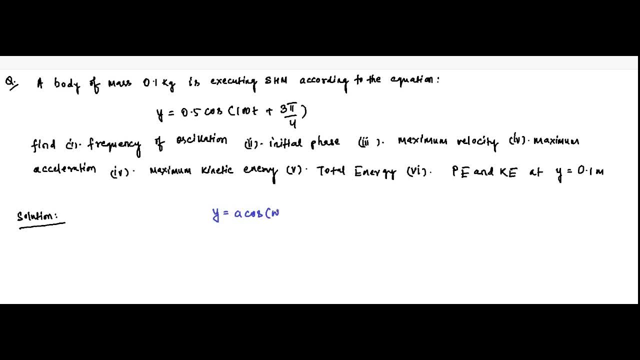 SHM equation is also in the format of cos, So it will be easy. So here y is equal to 0.5 into 0.2, into 2 by 4.. Here is the amplitude, Okay. So if we compare it with: 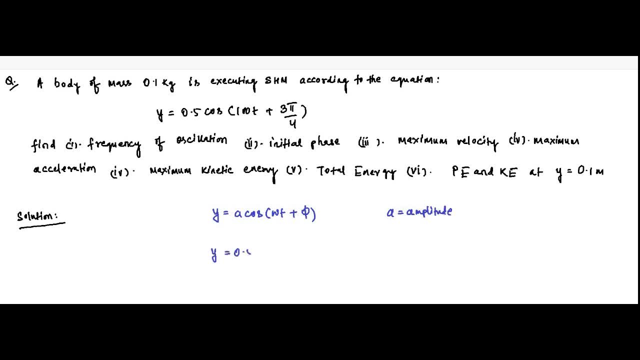 the given SHM equation, that is 0.5 cos 100 t plus 3 pi by 4.. If we compare it, then amplitude is equal to 0.5 meters. Yes, this is in meters. Okay, This much meters, Okay. So this is. 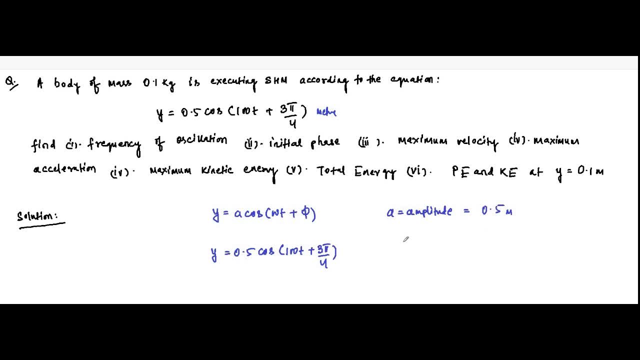 meter, Then angular frequency omega that is equal to 100 radians per second. Initial phase angle is equal to 3 pi by 4 radians. So this initial phase, second bit, we have already got initial phase angle, that is 3 pi by 4 radian. Then we know that angular frequency omega. 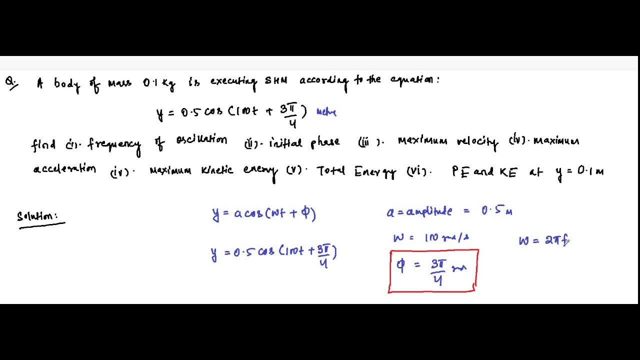 that is equal to 2 pi f, where f is frequency in hertz or second inverse. So frequency of oscillation, which is f, that is equal to omega, by 2 pi, which is equal to, here, 100 radians per second, by 2 pi, equal to 50 by pi hertz. So this is the frequency of oscillation that 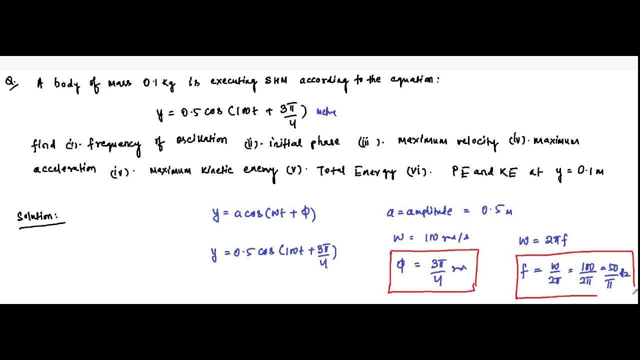 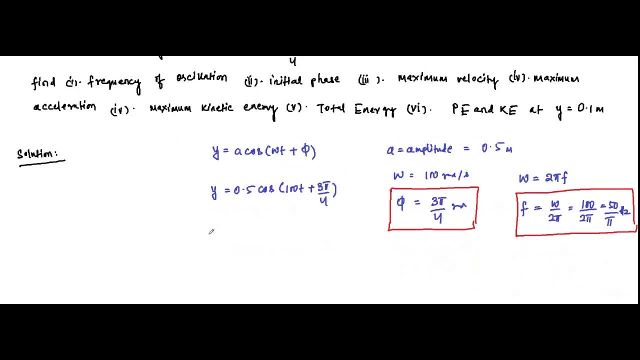 we have calculated. Then it has been asked to find the maximum velocity. So if you remember the maximum velocity in SHM 00.00, that is equal to omega, a omega angular frequency, a amplitude. omega is 100 radians per second. amplitude is 0.5, okay, meters. so it is how much? 50 meters per second? that is equal to v max, okay. 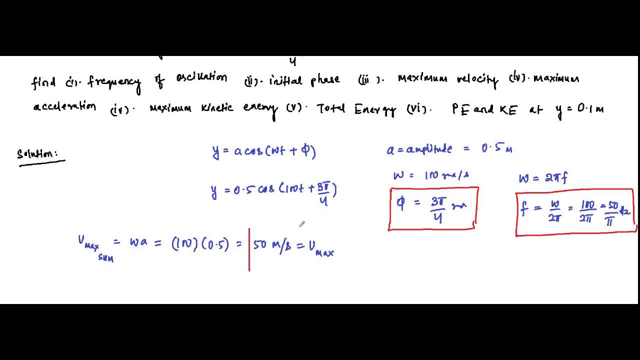 so this one we have calculated. then maximum acceleration, the acceleration maximum in shm, that is equal to omega square a. so again, basically it is omega square. that is how much 100 square into how much amplitude is 0.5. so that is equal to v max. okay, 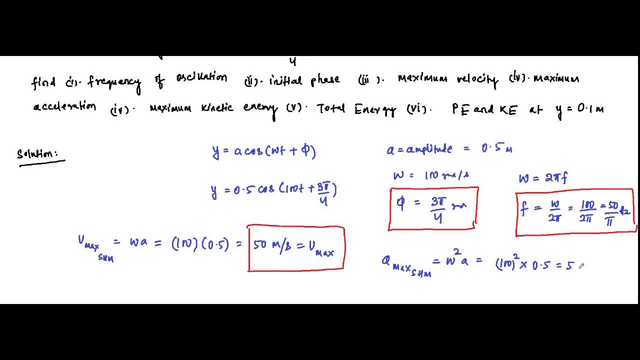 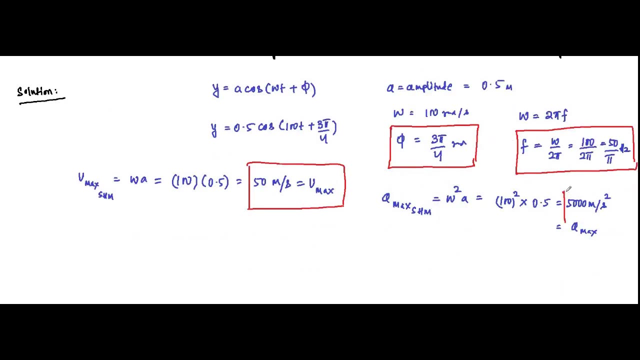 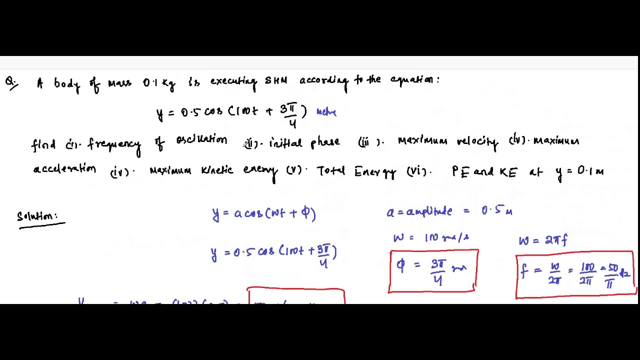 so that is equal to how much? 5000 meters per second square. so that is equal to the maximum acceleration. so that also we have calculated here, okay, this one. then it has been asked to determine the maximum kinetic energy. okay, kinetic energy, we have calculated here, okay. 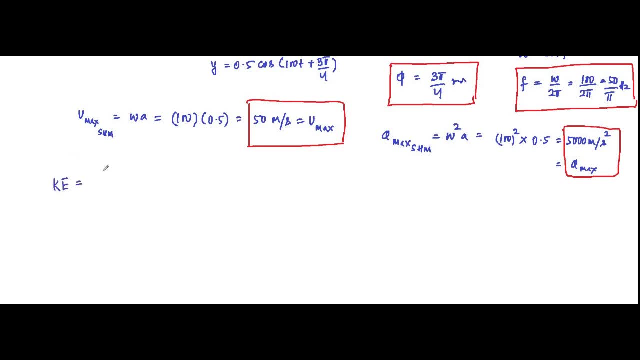 so this is the maximum kinetic energy. okay, kinetic energy we have calculated here. okay, so this is the maximum kinetic energy. okay, we all know for a mass m it is given by 1 half m v squared. so kinetic energy will become maximum when this velocity will be maximum. so 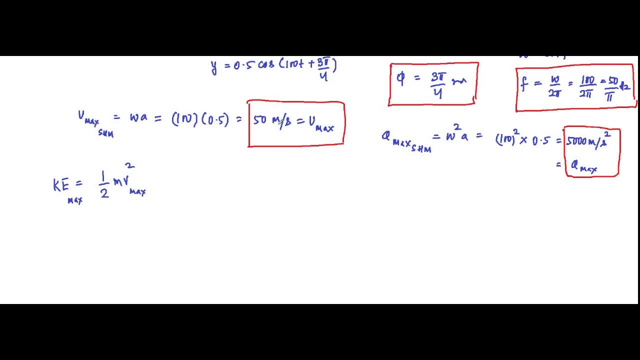 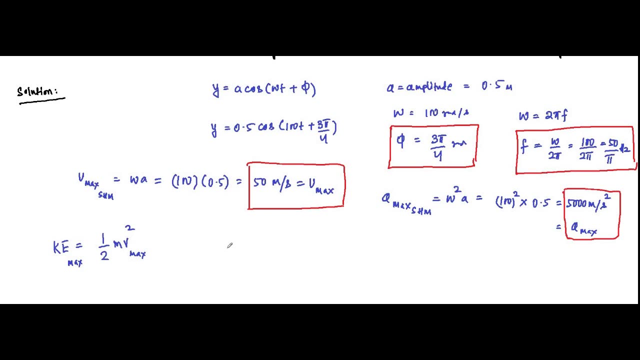 the maximum velocity for this SHM motion we have calculated is 50 meter per second. mass of the object is how much? 0.1 kg. okay, mass is 0.1 kg v max. we have already calculate 50 meter per second. simply will substitute the values into 0.1, into 50 whole. 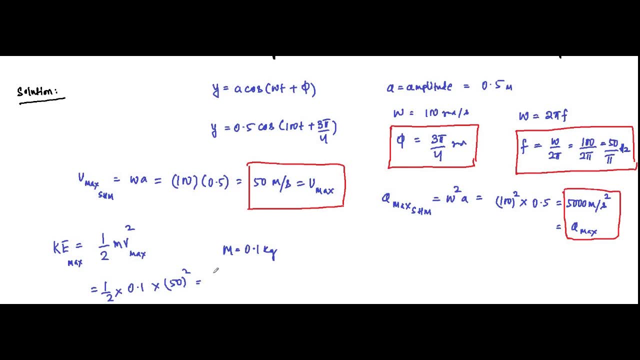 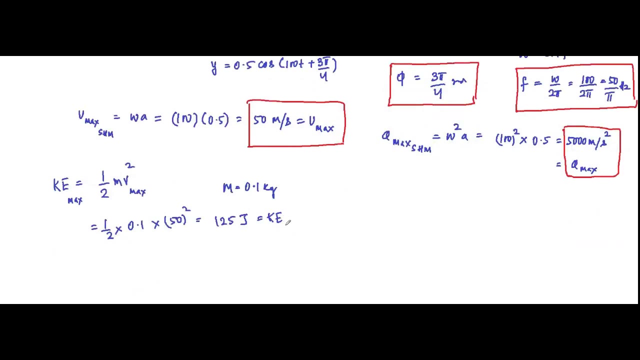 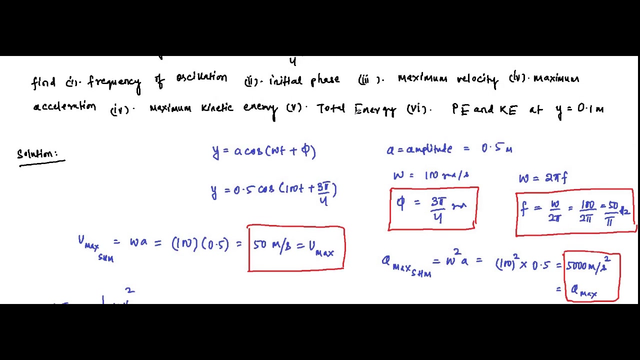 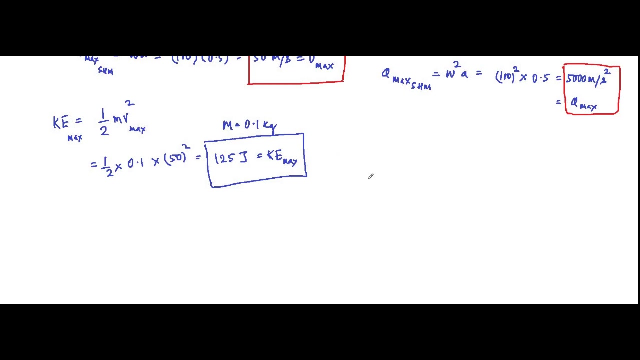 square that is equal to it is coming around 125 joules. So this is the maximum kinetic energy. okay, Now then it has been asked to find the total energy. Now see total energy. we can calculate using that k square minus y square, k that thing. 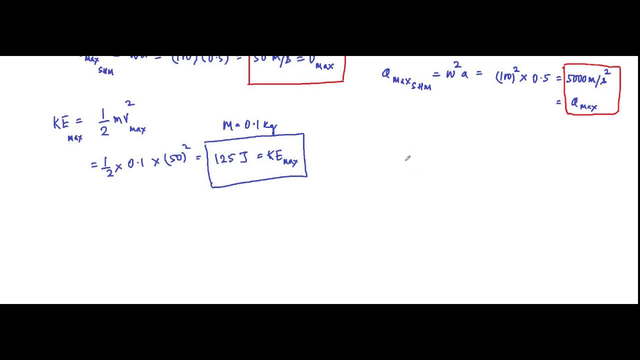 okay, Let us do it using that. we know that the kinetic energy, in terms of the instantaneous position of the object, that is given by 1 half k, a square minus y square. okay, A is the amplitude, y is the instantaneous position and k is the force constant for that. 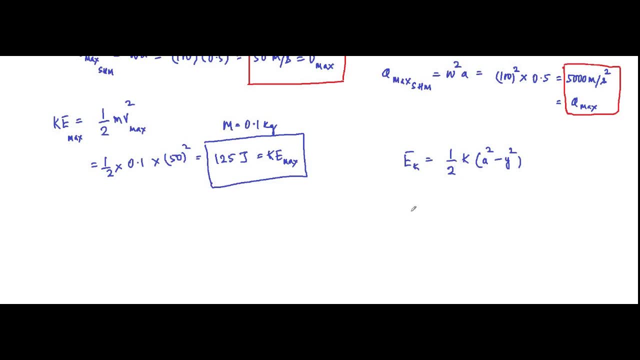 particular mass. Then the potential Total energy is given by 1 half k y square. Total energy is equal to kinetic energy plus potential energy. So this will be 1 half k square minus 1 half k y square plus 1 half k y square. 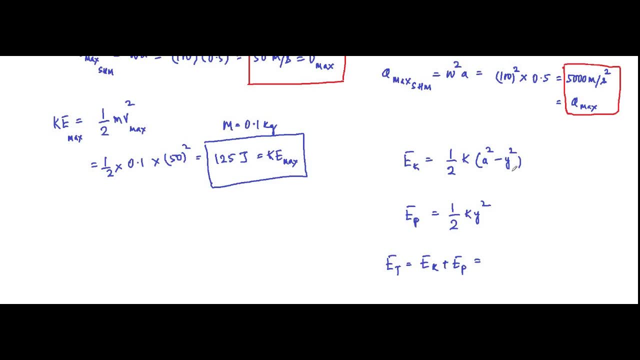 So this plus 1 half k y square and minus 1 half k y square, that will get cancelled. So it will be simply 1 half k a square. So here k we will calculate. We know that the angular frequency omega is equal to root over of k by m. 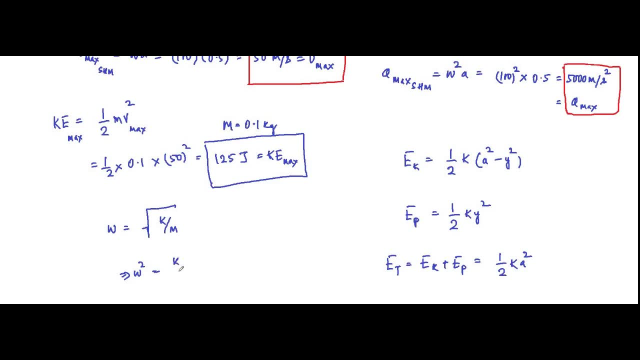 That implies omega square is equal to k by m. That implies k is equal to m omega square, which is equal to how much? 0.1 kg. mass. Angular frequency is 100 radians per second, So that becomes how much? 1000 newton per meter. 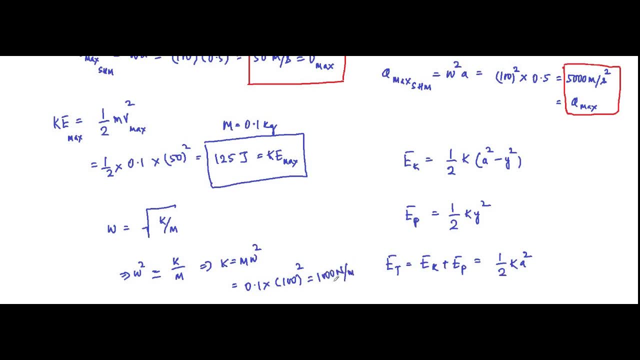 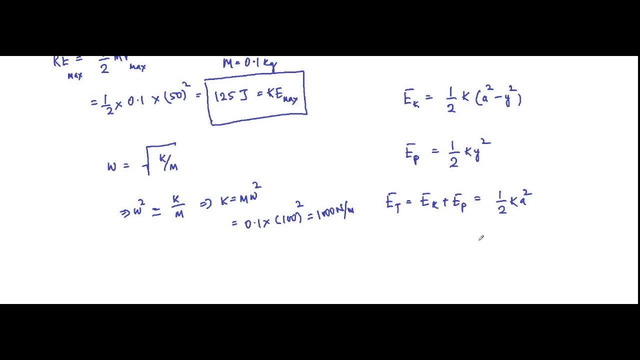 This is the value of k, the force constant. So here, simply, we will substitute the value. This is equal to the total energy: 1 half k, which is equal to 1000 Newton per meter. This is equal to k, which is equal to 2000 Newton per meter. 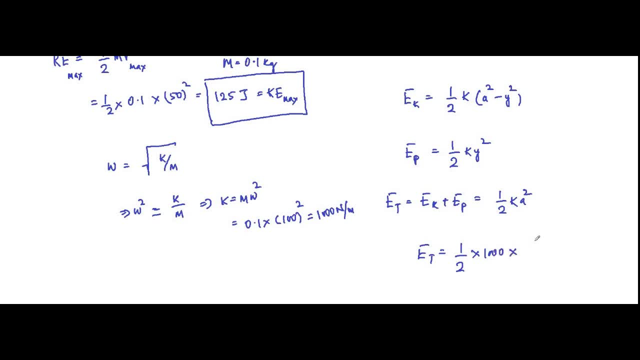 So the force constant is 0.1 kg mass And A is the amplitude, which is equal to 0.5 meter, that is, 0.5 whole square. So this is coming around 125 joules. that is the total energy. 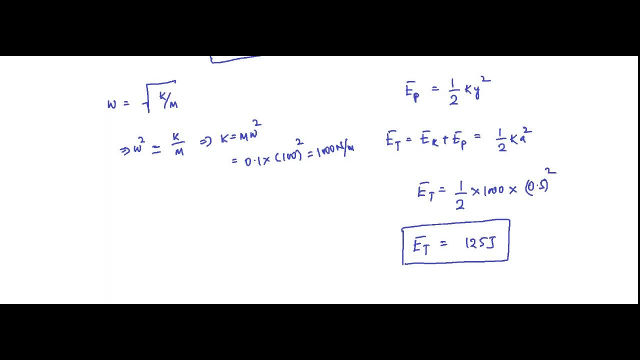 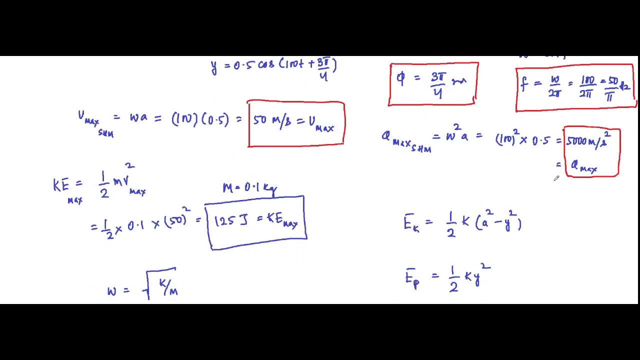 Okay, this, that is the total energy here, This, Okay, we will discuss some important thing, Okay, but later. first let us calculate this potential energy. and kinetic energy at y is equal to 0.1 meter, So here we will substitute the value. 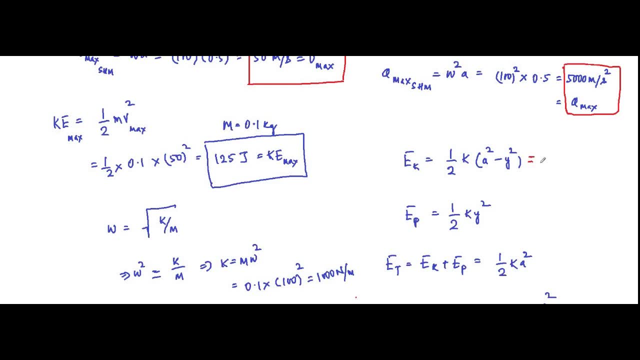 So kinetic energy at y is equal to 0.1 meter, So it is one half into 1000. the force constant A is 0.5 whole square minus y, Which is 0.1 whole square. So that is coming around 120 joules. 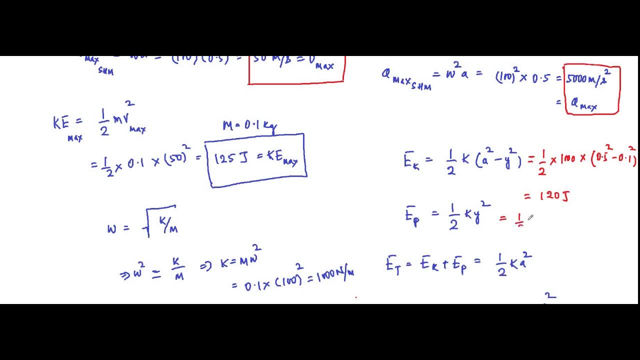 And here potential energy one half into 1000, into y, Which is 0.1 whole square, that is equal to 5 joule. Okay, So potential energy and kinetic energy at y is equal to 0.1 meter. 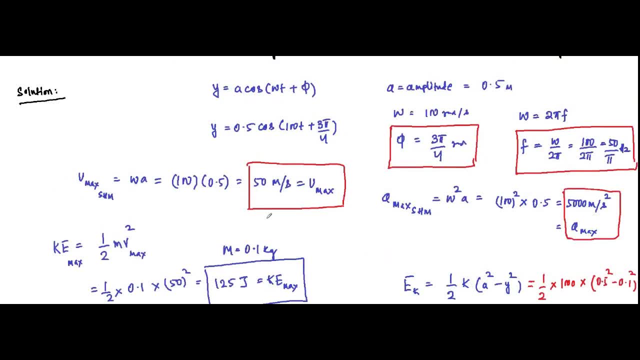 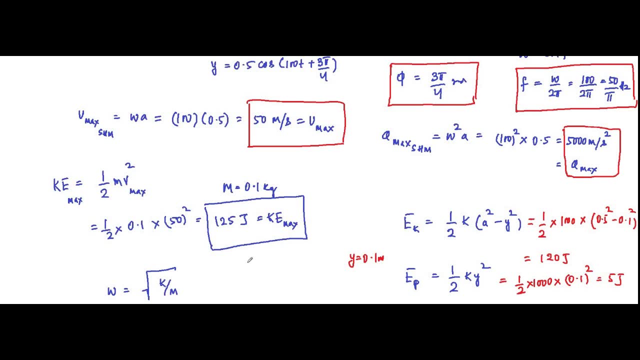 Okay, Now see here we calculated the maximum kinetic energy. Maximum kinetic energy occurs when potential energy is equal to 0.. Okay, And maximum kinetic energy that is equal to 125 joule. Sum is equal to 125 joule.